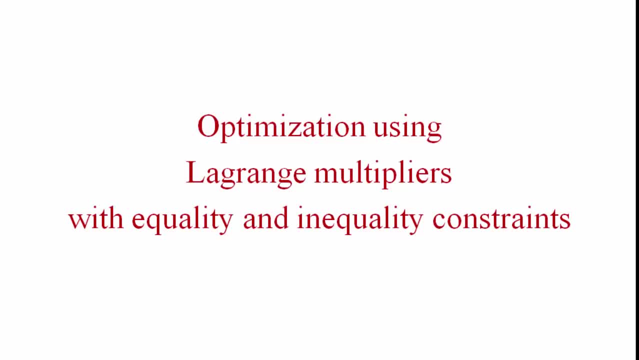 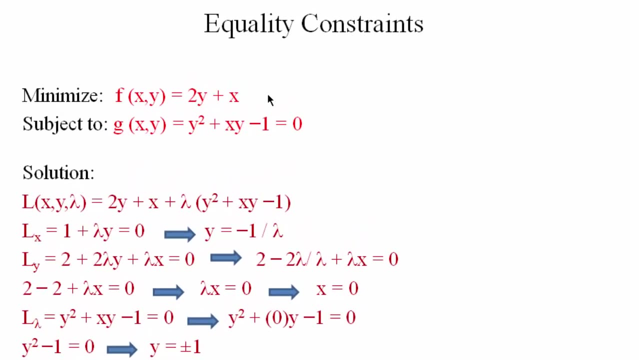 Hello and welcome. I'm going to show how to optimize a function using Lagrange multipliers with equality and inequality constraints. In this example, we want to minimize this function, which is a function of two variables, x and y, 2y plus x, And this is the constraint. 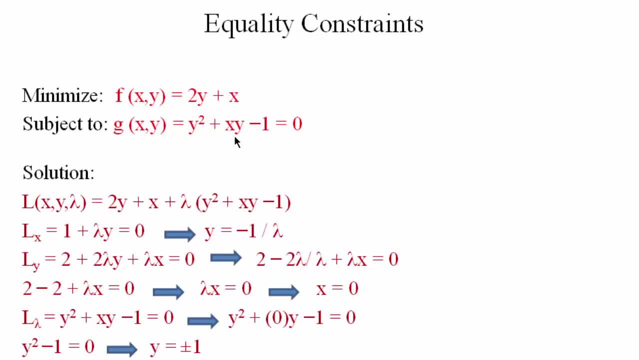 which is also a function of x and y. First of all, we're going to write the objective function and the constraint in a single equation, which is this one. So this function, L, is a function of x, y and lambda Lambda here is called the Lagrange multipliers. 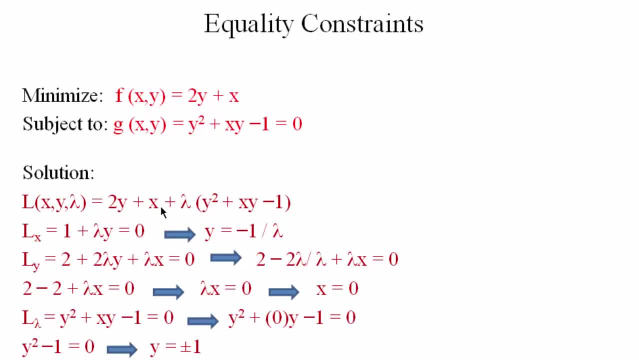 So this is the objective function: 2y plus x plus lambda, the Lagrange multiplier multiplied by the constraint, which is y squared plus xy minus 1.. Notice that if we have a constant here, for example if we have the number 5 here, then we have to move this 5 to the left. 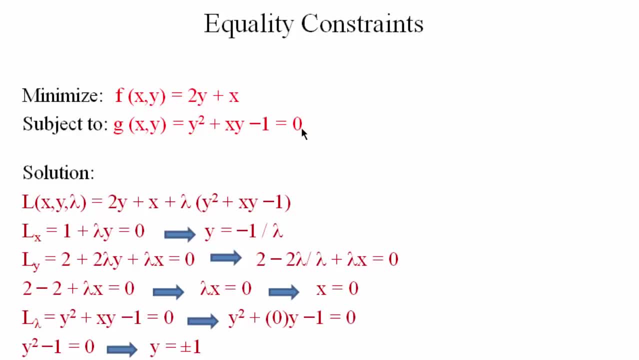 side of the equation and make the equation equals 0.. Now we're going to differentiate this equation with respect to x, y and lambda. So when we differentiate with respect to x, we get 1, plus lambda here will be distributed to: 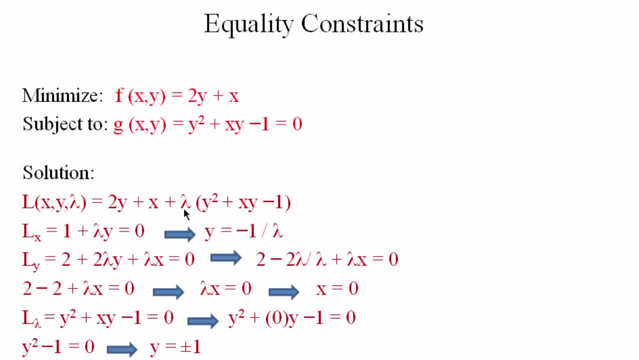 all the three terms And when we differentiate we'll get lambda y for this term. Now we're going to add 2y plus lambda and we make the equation equal to 0, and we find this equation: When differentiating with respect to y, we get 2 from here because of the two 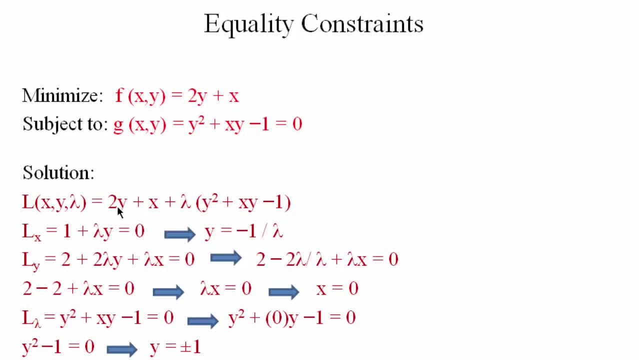 y in the equation, when we differentiate with respect to y, we get 2, plus this will be 0, to the other term, 2y, And this lambda will be distributed here and here Lambda y square will be 2 lambda y. 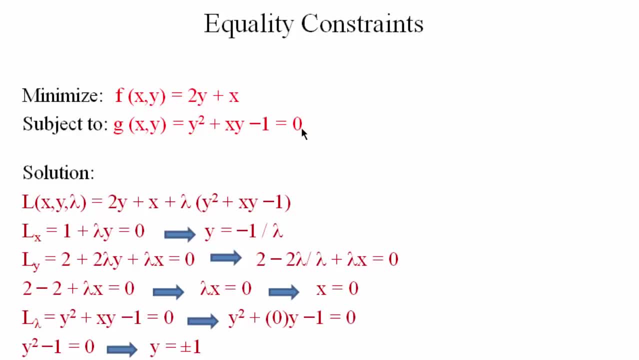 side of the equation and make the equation equals 0.. Now we're going to differentiate this equation with respect to x, y and lambda. So when we differentiate with respect to x, we get 1, plus lambda here will be distributed to: 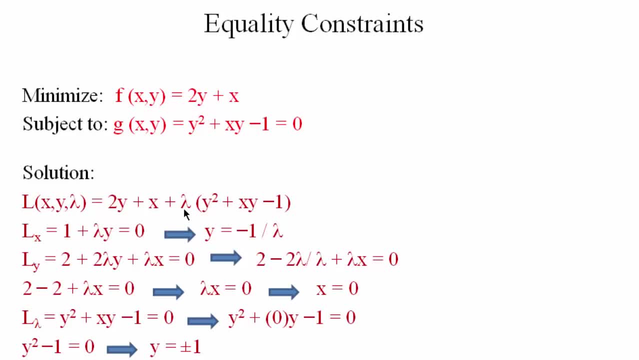 all the three terms And when we differentiate we'll get lambda y for this term. Now we're going to haveер we infinite w, e and val and we make it equal to 0. And we find this equation: When differentiating with respect to y, we get 2 from here, because 2y when 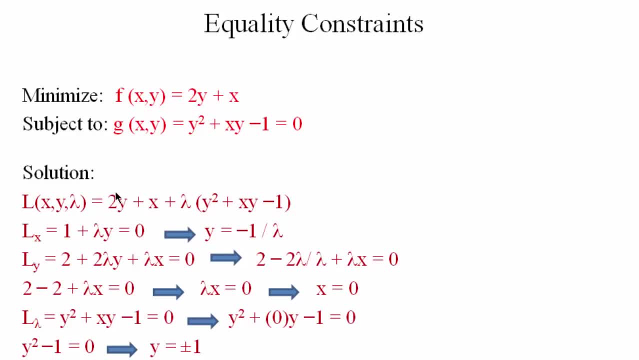 we differentiate with respect to x, y, we get 2.hou 7, plus 1,. we multiply by the constraints, we find 2.. And when we differentiate with respect to y, we get comm ί, which is almost 2.. Plus, So we get 2, because when we differentiate with respect to y, we get 2.. Well, we can always Print bars for relativeematic angles. So from our Cant ignorance, how many we have obtained. So the derivative function empty cell punto ez will give us equal to 0 select. 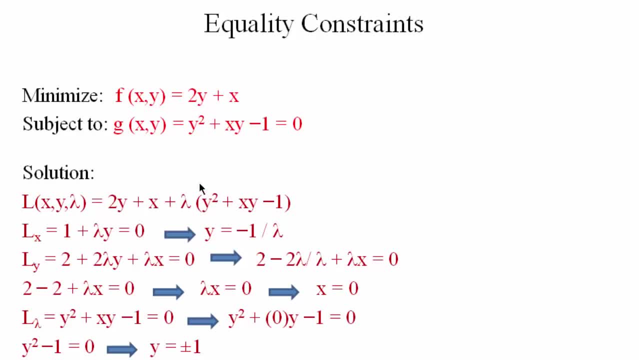 with respect to y 15, but we know that 5 plus simple жен is present in several And this lambda will be distributed here and here. Lambda y square will be 2, lambda y And lambda xy will be lambda x equals 0.. And we get this equation Which leads to x equals 0.. 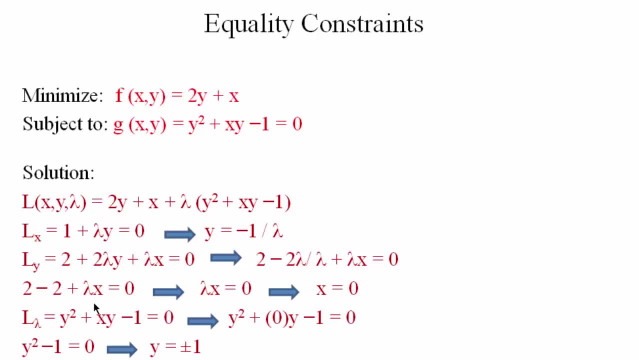 Finally, we differentiate the equation with respect to lambda, So we get this equals 0, this equals 0.. And when we differentiate this term, we get y square plus xy minus 1.. Which is this equation Equals 0.. And since we have x equals 0 from ly, we substitute x equals 0.. 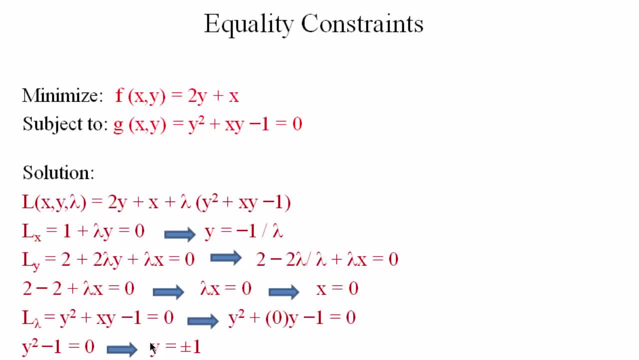 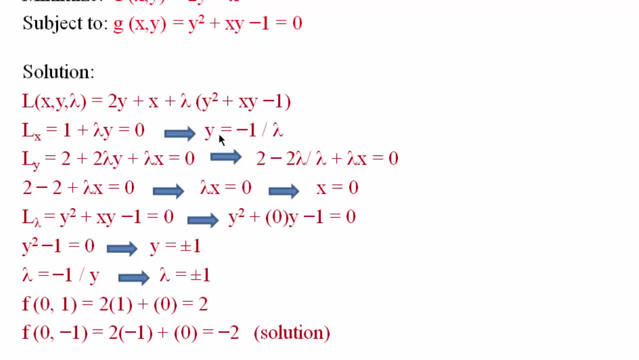 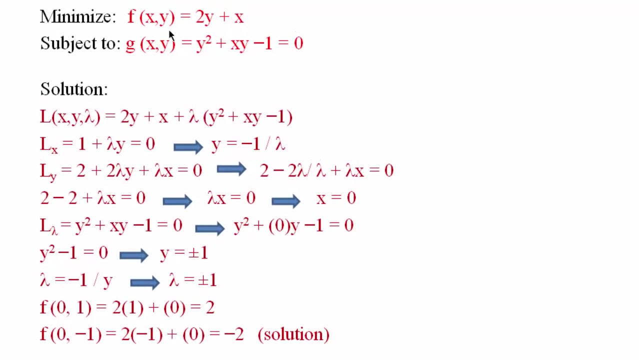 And this equation And we get y equals plus minus 1.. And from this, y equals plus minus 1, if we substitute here, we get lambda, Which equals to plus minus 1.. Now we have the values of x and y, Which are the important variables that we need to minimize our function. 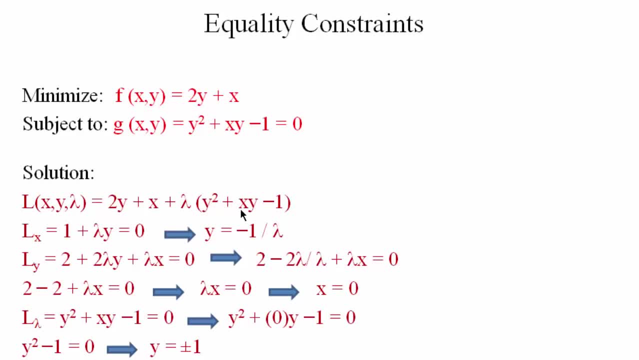 And lambda xy will be lambda. x Equals 0.. And we get this equation Which leads to x equals 0.. Finally, we differentiate the equation with respect to lambda, So we get this equals 0, this equals 0. 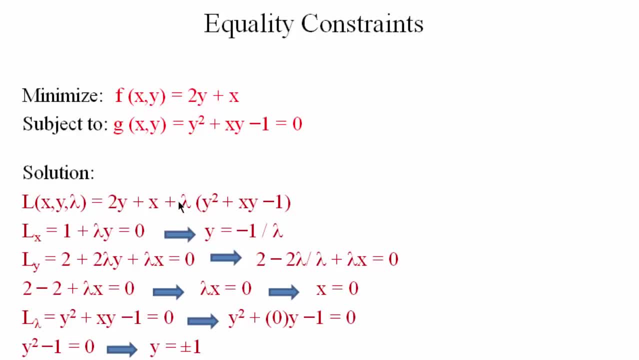 And when we differentiate this term, we get y square plus xy minus 1.. Which is this equation Equals 0.. And since we have x equals 0 from ly, We substitute. We substitute x equals 0 in this equation And we get y equals plus minus 1.. 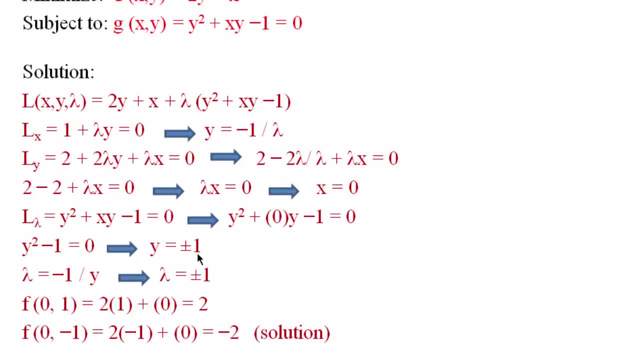 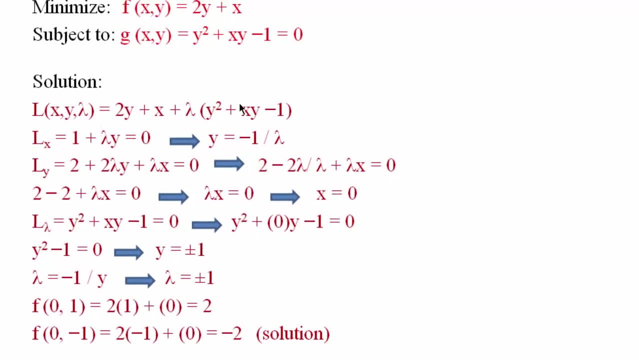 And from this y equals plus minus 1.. If we substitute here, We get lambda, Which equals to plus minus 1.. Now we have the values of x and y, Which are the important variables that we need to minimize our function. 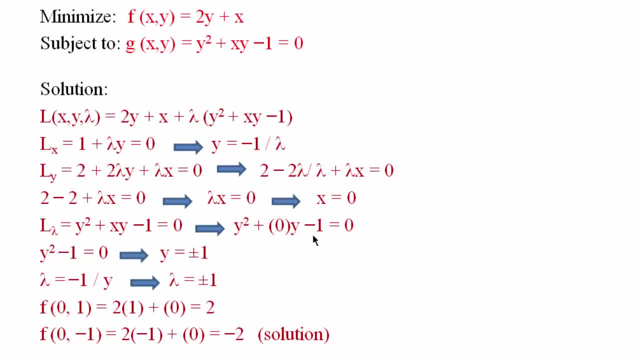 Now we just need to test these numbers First that we obtained x equals 0 and y equals plus minus 1.. So we are going to substitute: x equals 0 and y equals 1.. x equals 0 and y equals minus 1.. 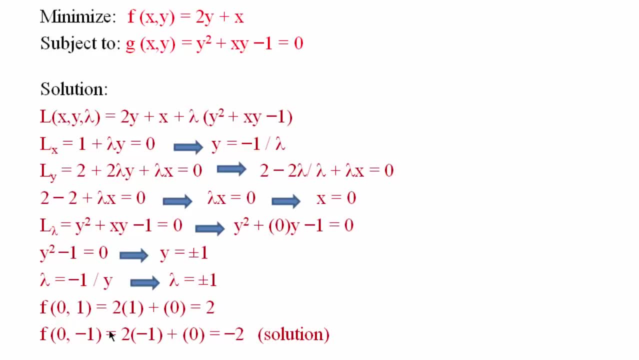 And from these values we get f equals 2.. And from these values we get f equals minus 2.. So we have 2 and minus 2.. The minimum is minus 2.. Because we want to minimize the function. 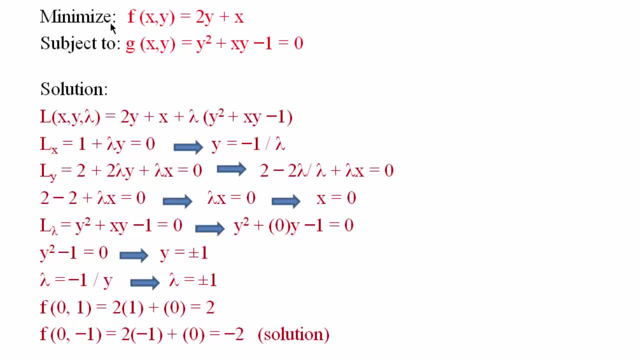 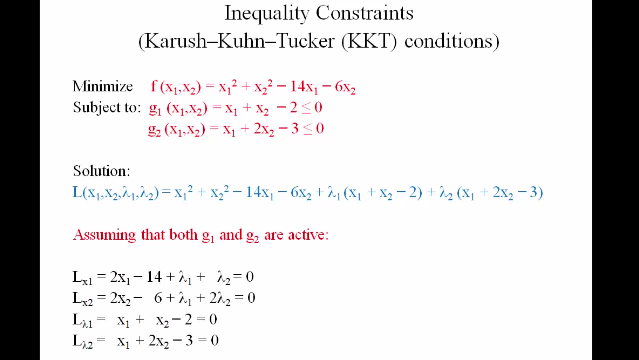 Which means that the values of x And y- That minimizes the function- Is 0 and minus 1.. Now let's talk about the inequality constraints. We are going to use the Lagrange multipliers as well. However, we are going to test some conditions. 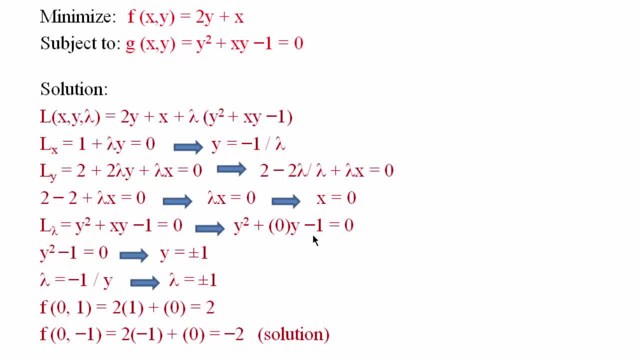 Now we just need to test these numbers that we obtained. So we are going to substitute x equals 0 and y equals plus minus 1.. So we are going to substitute x equals 0 and y equals 1.. x equals 0 and y equals minus 1.. 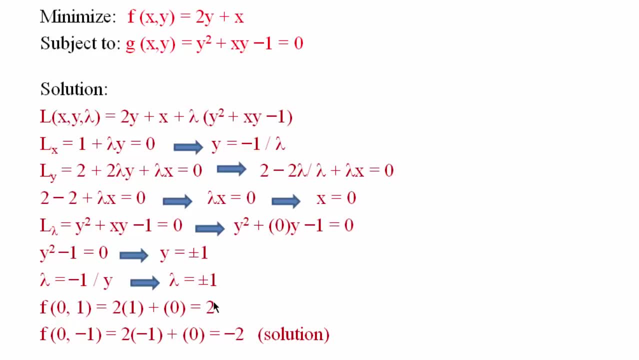 And from these values we get f equals 2.. And from these values we get f equals minus 2.. So we have 2 and minus 2.. The minimum is minus 2.. Because we want to minimize the function. 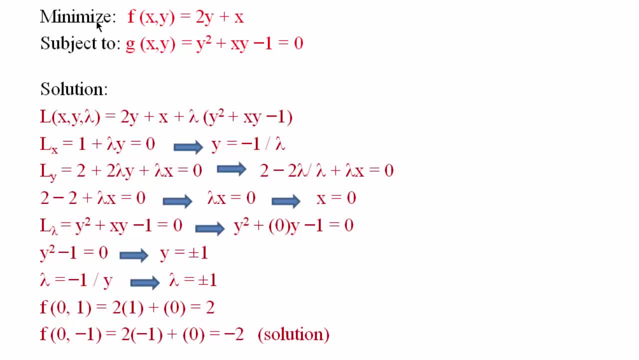 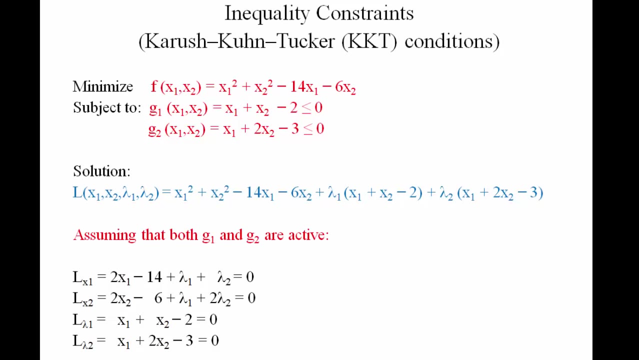 Which means that the values of x and y, Which minimizes the function- Is 0 and minus 1.. Now let's talk about the inequality constraints. We are going to use the Lagrange multipliers as well. However, we are going to test some conditions. 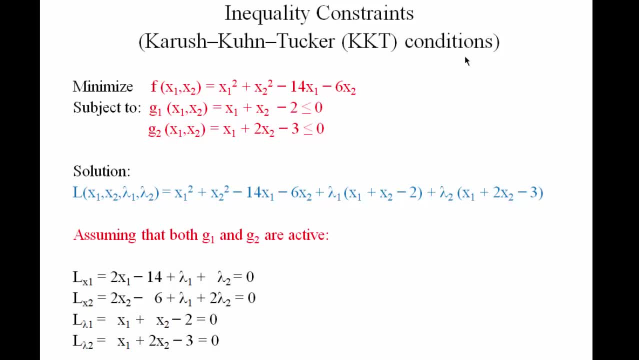 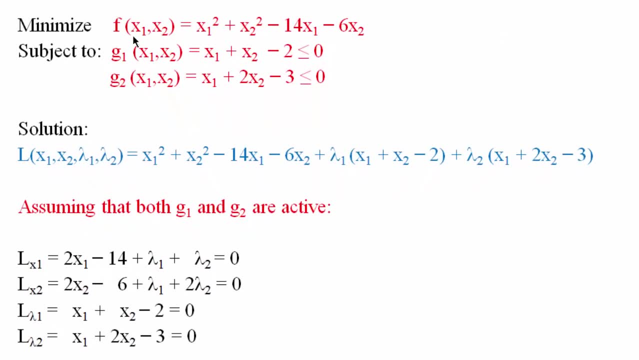 Which are called the KKT optimality conditions. Let's minimize this function. This function has two variables- x1 and x2, and we have two constraints, g1 and g2.. These constraints are inequality constraints. Similar to what we did in the previous example. we are going to write one equation that collects all variables: x1, x2, lambda1, and lambda2.. 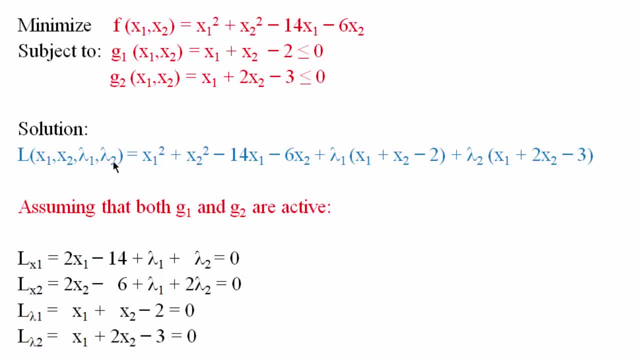 Lambda1 and lambda2 are the Lagrange multipliers. Therefore we write the objective function here, which is this one plus lambda1 multiplied by the first constraint, which is this one plus lambda2 multiplied by the second constraint, which is this one: 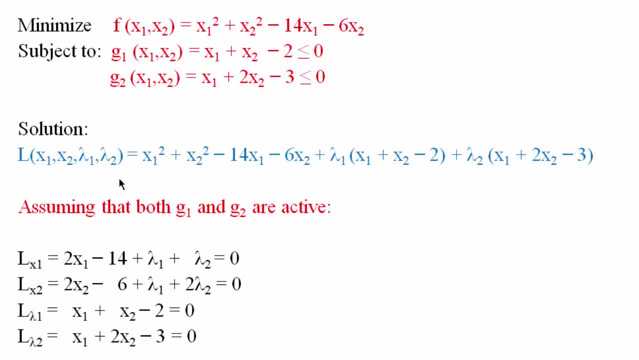 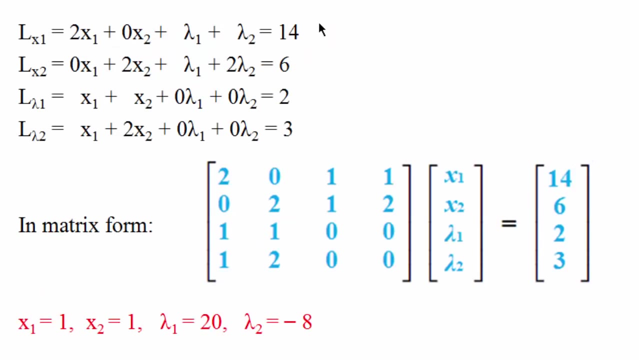 As we did in the previous example, we differentiate this equation with respect to x1, with respect to x2.. So we have lambda1 and lambda2.. So we have four equations Here. I have just rewritten the four equations in this way. 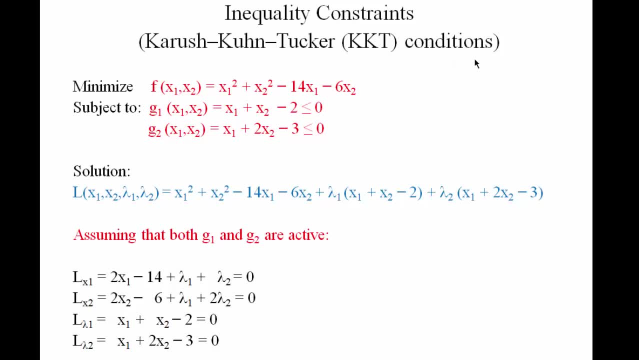 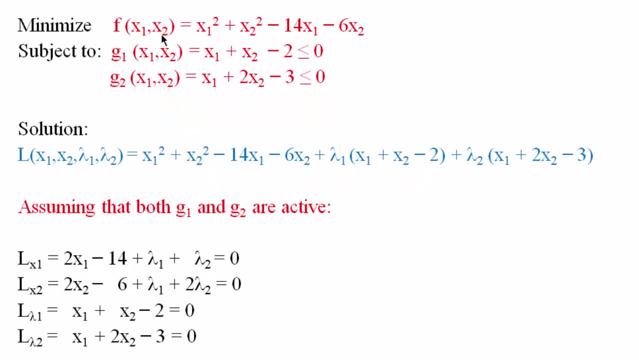 Which are called the KKT optimality conditions. Let's minimize this function. This function has two variables, x1 and x2.. And we have two constraints: g1 and g2.. These constraints are inequality constraints, Similar to what we did in the previous example. 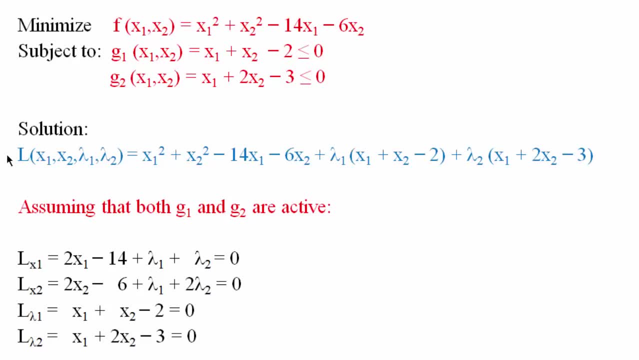 We are going to write one equation That collects all variables x1, x2, lambda1 and lambda2.. Lambda1 and lambda2 are the Lagrange multipliers. Therefore we write the objective function here, Which is this one: 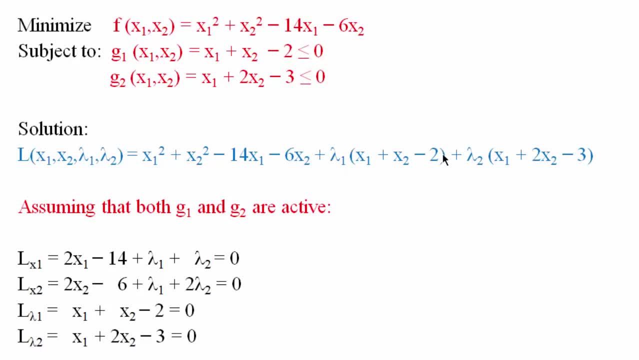 Plus lambda1 multiplied by the first constraint, Which is this one. Plus lambda2 multiplied by the second constraint, Which is this one: As we did in the previous example, We differentiate this equation with respect to x1.. With respect to x2.. 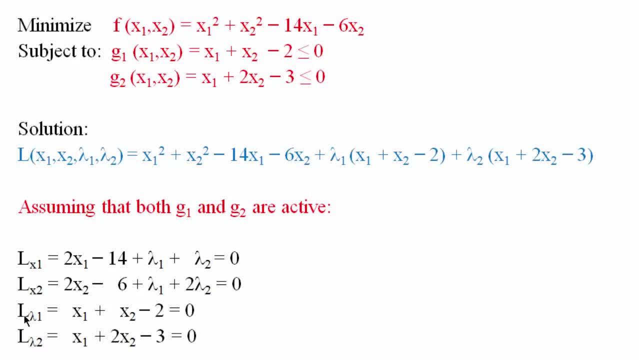 With respect to x3.. Lambda1: With respect to x3.. With respect to x5.. With respect to x6.. With respect to x6.. With respect to x9.. With respect to x8.. With respect to x10.. With respect to x11.. 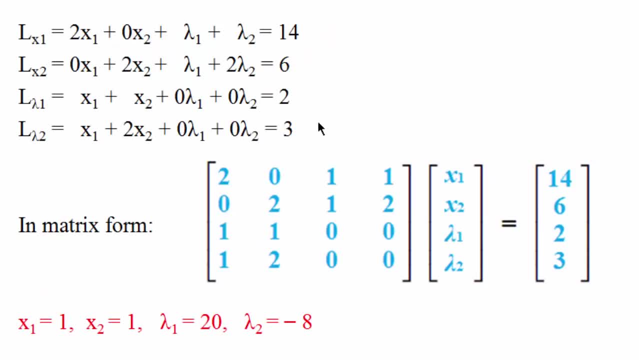 With respect to x14.. With respect to x13 and x15.. With respect to x14. We have a values of lambda1 and lambda2.. So we have four equations Here. I have just trialten the four equations And this way: 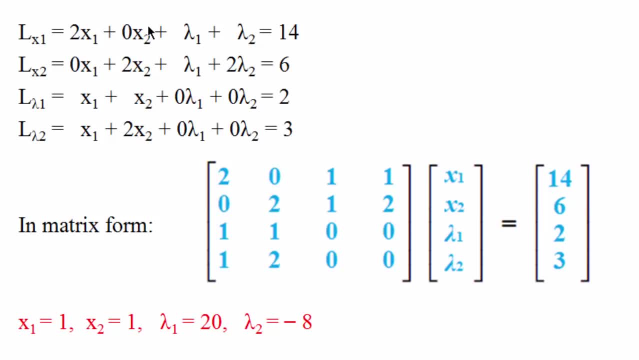 So I added all variables x1,, x2.. We don't have x2 in the first equation, So I added zero, x2, lambda1, and lambda2.. Here also we have zero. x1길 대비 X₁. 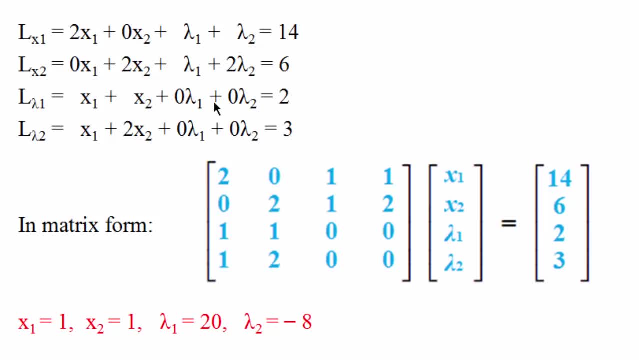 X₂- lambda1 and lambda2.. X₂- lambda1 and lambda2.. x1, x2, 0 lambda 1 and 0 lambda 2, and so on. we can write these four equations in a matrix form, so these numbers here represent the coefficients of the 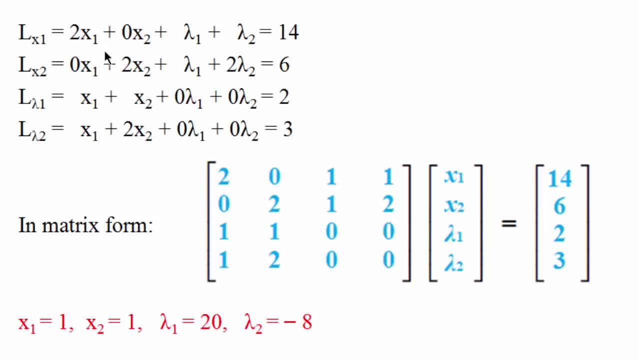 variables. so this 2 represents the coefficient of x1, 0 represent the coefficient of x2, 1 represents the coefficient of lambda 1 and 1 represent the coefficient of lambda 2. so this is the first row and this is x1, x2, lambda 1. 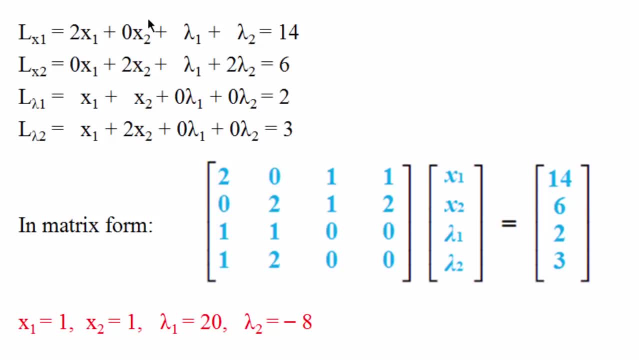 So I added all variables x1,, x2.. We don't have x2 in the first equation, so I added 0,, x2,, lambda1, and lambda2.. Here also we have 0,, x1,, x2,, lambda1, and lambda2.. 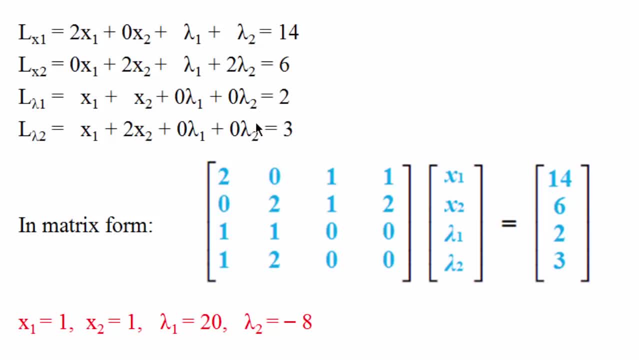 Here also we have 0, x1, x2,, 0, lambda1, and 0, lambda2, and so on. We can write these four equations in a matrix form. So these numbers here represent the coefficients of the variables. 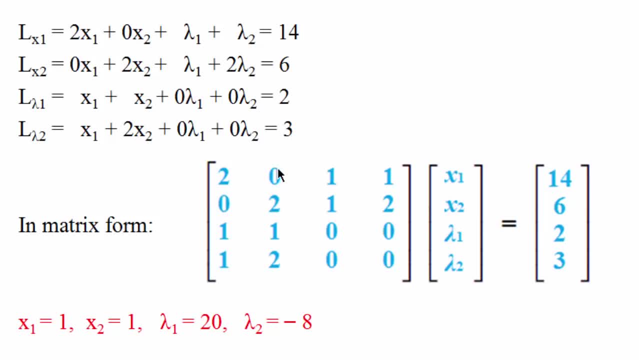 So this 2 represents the coefficient of x1.. 0 represents the coefficient of x2.. 1 represents the coefficient of lambda1.. And 1 represents the coefficient of lambda2.. So this is the first row And this is x1.. 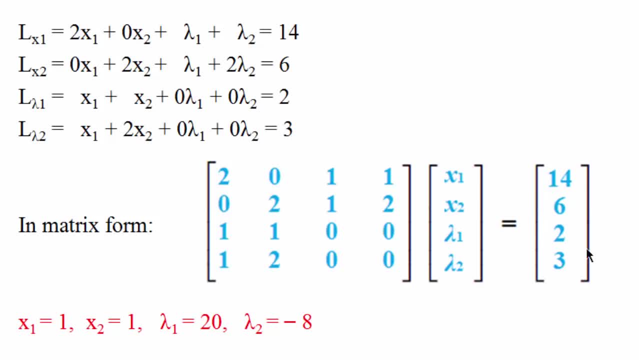 x2,, lambda1, and lambda2.. And these are the constants, which are 14,, 6,, 2, and 3.. Also, this row represents the coefficients of the second equation: 0,, 2,, 1, and 2.. 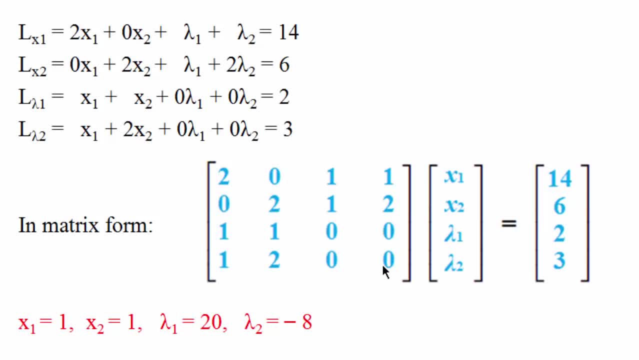 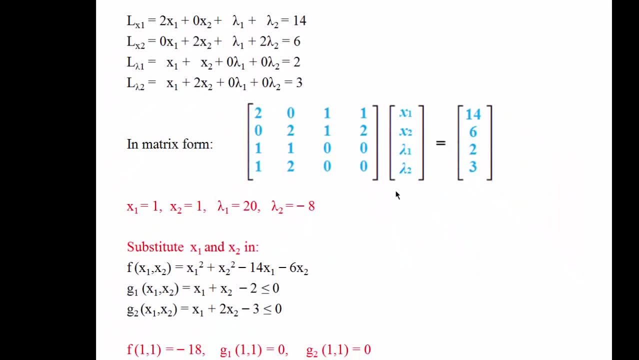 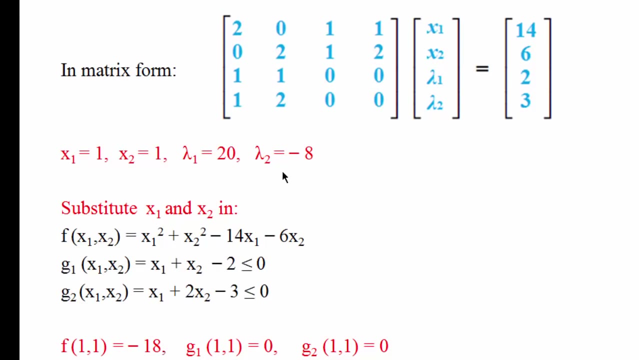 And so on for the third and the fourth equations. Now we can simply solve this problem to find x1, x2, lambda1, and lambda2, which gives these results. Now we need to test these results by substituting in the objective function, which is this one: 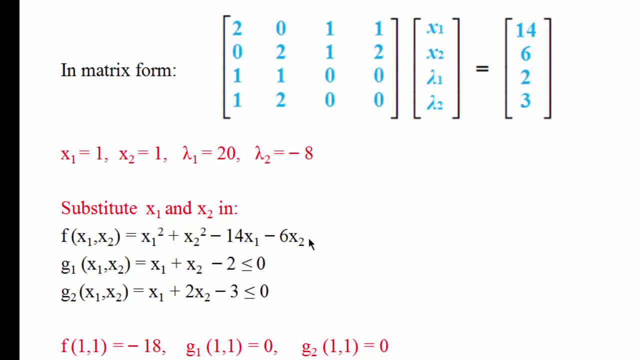 I have just rewritten the objective function as given in the example And these are the two constants as given in the example, And by substituting the values of x1 and x2 in the objective function and the constants we get the function. f equals minus 18.. 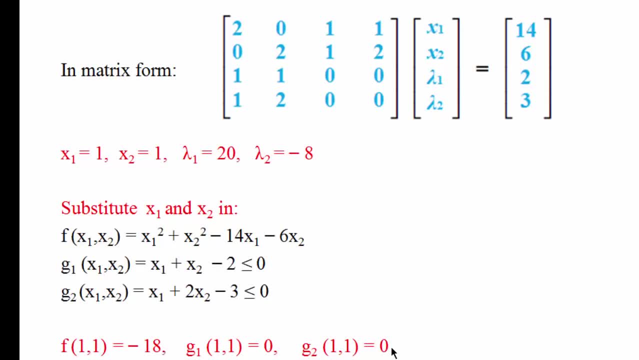 g1 equals 0, and g2 equals 0. Since both constants are less than or equal to 0, then we have no problems with the constants And we have this value, which should be the minimum value. However, since one of the Lagrange multipliers has a negative value, 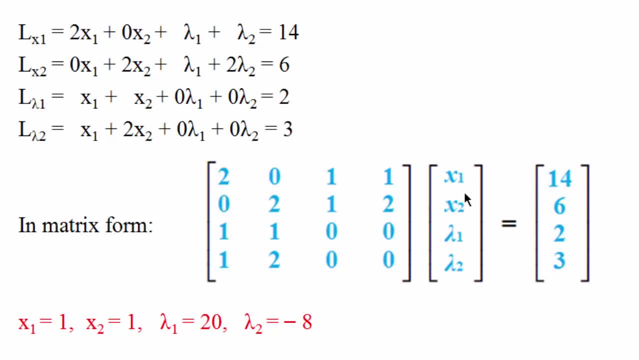 and lambda 2, and these are the constants, which are 14, 6, 2 & 3. also, this row represents the coefficients of the second equation: 0, 2, 1 & 2, and so on for the third and the fourth equations. now we can simply solve this problem to: 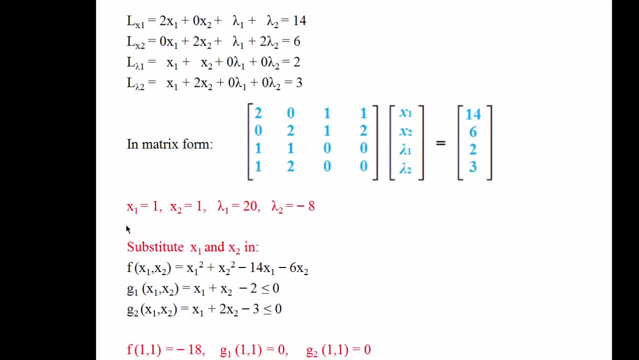 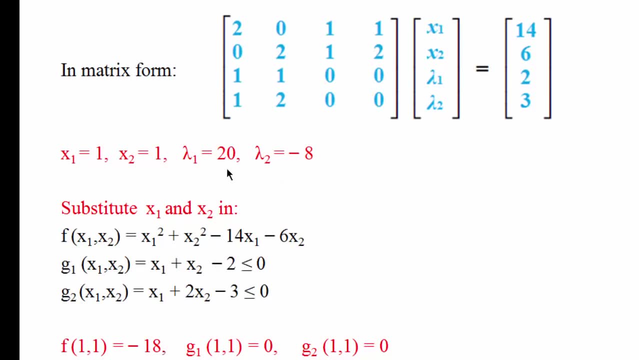 find x1, x2, lambda 1 and lambda 2, which gives these results. now we need to test these results by substituting in the objective function, which is this one- I have just rewritten the objective function as given in the example and these are the two constants as given in the example- and by substituting the 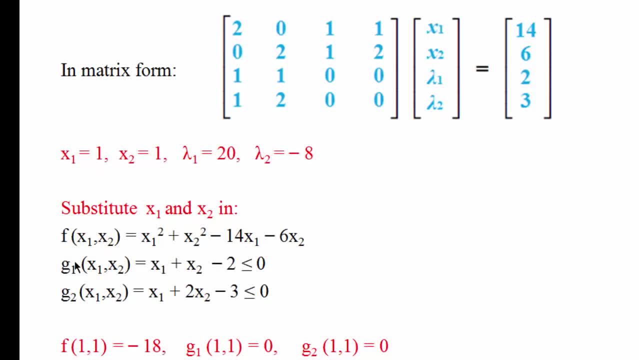 values of x1 and x2 in the objective function and the constraints, we get the function. f equals minus 18, g1 equals 0 and g2 equals 0. since both constraints are less than or equal to 0, then we have no problems with the constraints and we have this value. 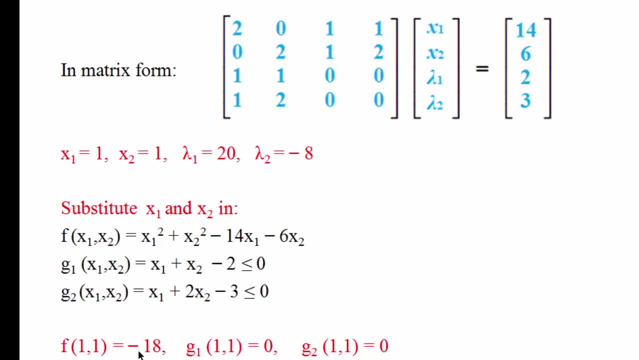 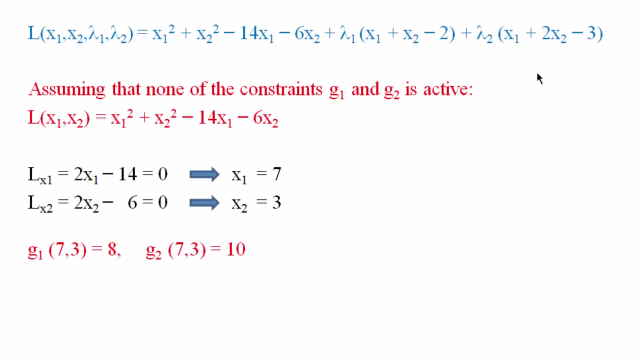 which should be the minimum value. however, since one of the Lagrange multipliers has a negative value, this means that this solution is not the optimal based on KKT optimality conditions. therefore, we are going to make another assumption. let's assume that none of the constants g1 and g2 is active, so from 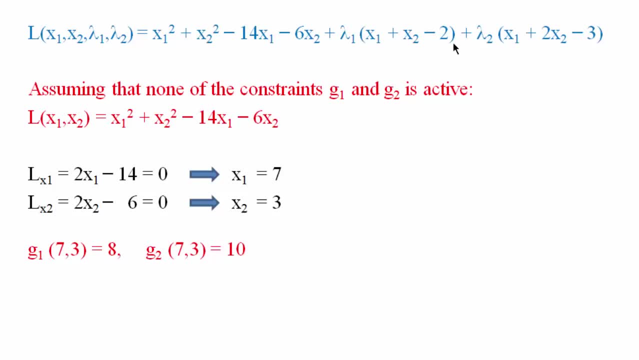 this equation. we are going to discard this term and this term and we have only this equation, which has only the objective function. now we differentiate the equation with respect to x1 and x2 and we get two equations. we have x1 equals 7, x2 equals 3. now, to test these values, we need to substitute them in the 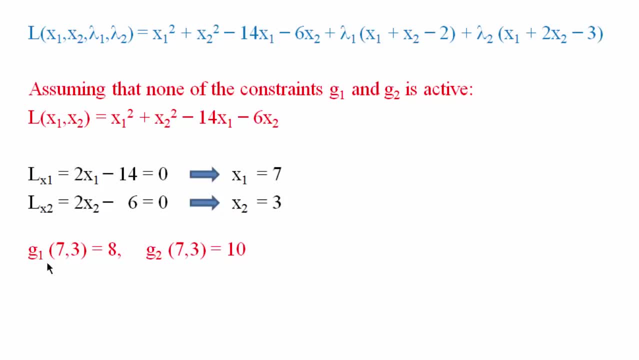 constraints function. so we have g1 equals 1: 1 and g2 equals 3. this equals g1: 8 and g2 equals 10. we can see that both g1 and g2 have positive values, which is not acceptable, because each of the constraints has an equality of less than 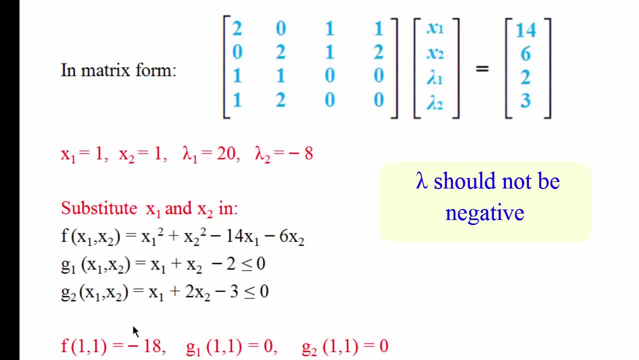 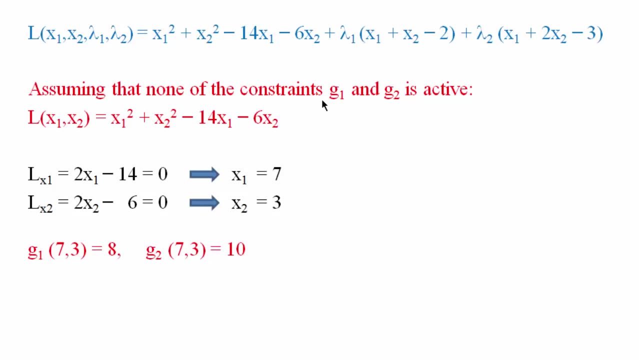 this means that this solution is not the optimal. Therefore, we are going to make another assumption. Let's assume that none of the constants g1 and g2 is active, So from this equation, we are going to discard this term and this term. 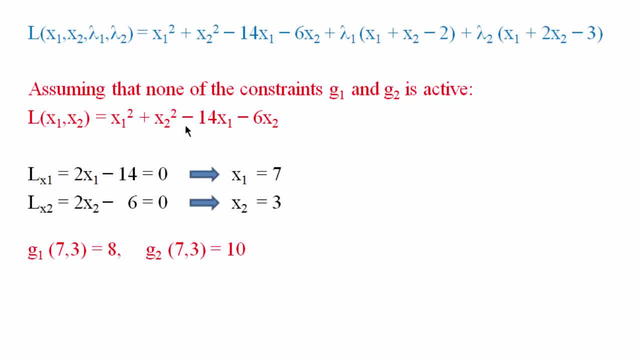 And we have only this equation, which has only the objective function. Now we differentiate the equation with respect to x1 and x2.. And we get two equations. We have x1 equals 7, x2 equals 3.. Now to test these values, we need to substitute them in the constraint functions. 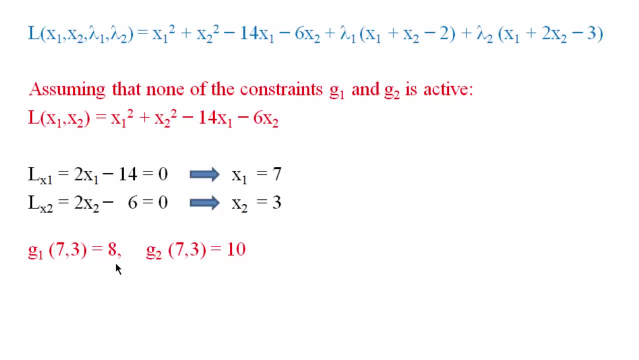 So we have: g1 equals 8 and g2 equals 10.. We can see that both g1 and g2 have constants And we have positive values, which is not acceptable because each of the constants has an equality of less than or equal to 0.. 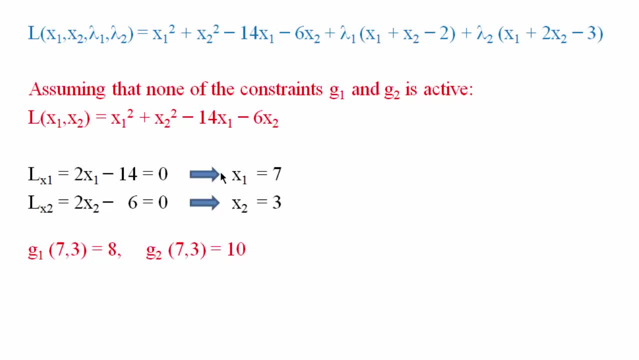 And since we have positive values here, which means that these values of x1 and x2 are not acceptable for a solution. Now let's do another assumption. We are going to assume that only g1 is active, Which means that we are going to assume that only g1 is active. 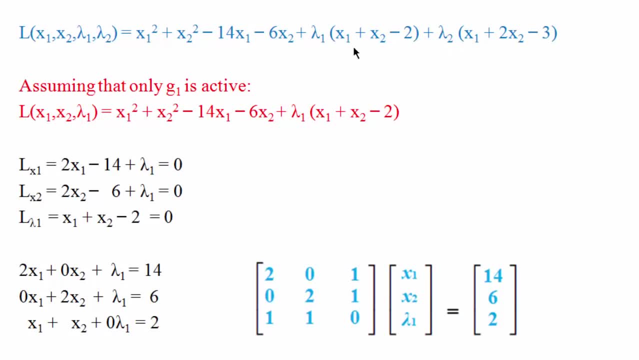 Which means that we are going to assume that only g1 is active, And now we are going to discard this term And we keep only this equation, which is the objective function and the first constant in this equation. Similarly, we are going to differentiate against with respect to x1, x2 and lambda-1. 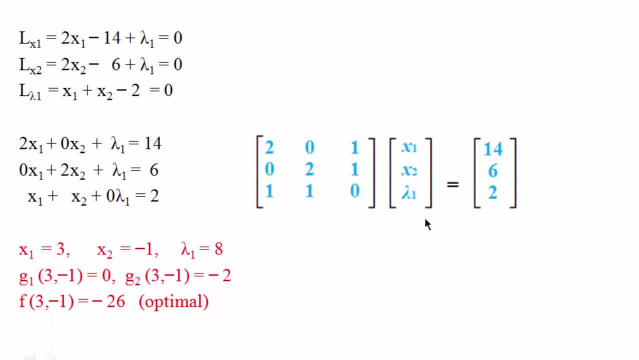 Here we rearrange the equations and the matrix form So we can solve easily to find x1, x2 and lambda-1.. lambda 1: now let's test the values by substituting in g1, which gives 0, which is acceptable, and g2 is minus 2, which is also acceptable, and by substituting in: 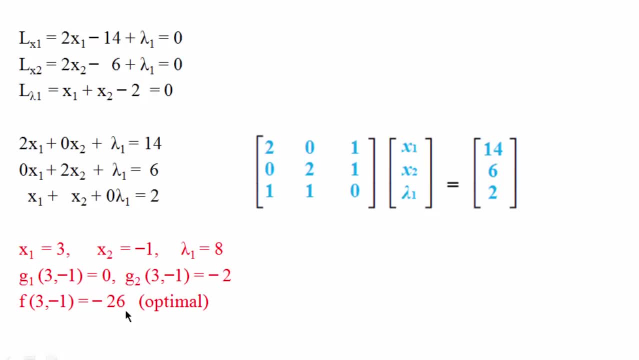 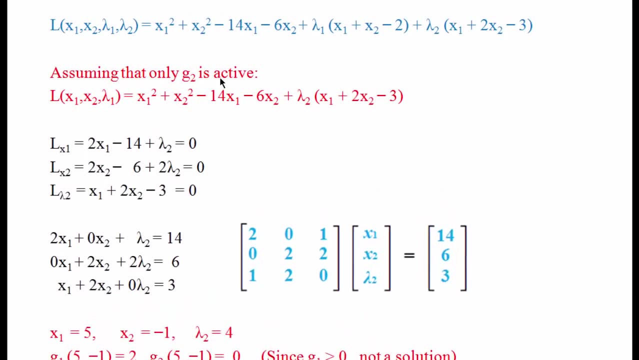 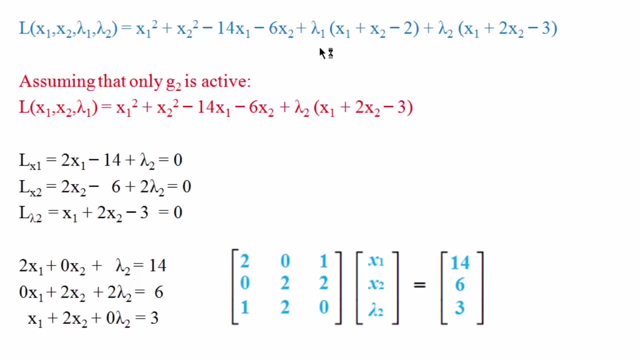 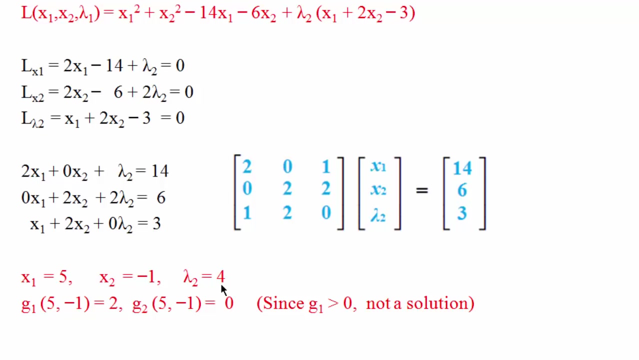 the objective function, we get the optimal result, which is minus 26. we can make one further assumption by assuming that only g2 is active. therefore we are going to discard this term and we'll keep this in the equation. now we are going to follow the same steps to find x1, x2 and lambda 2, and by substituting 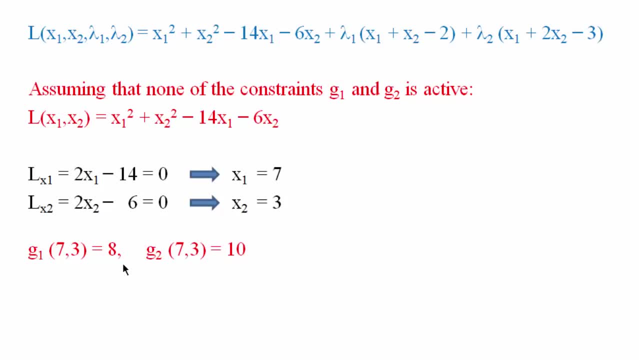 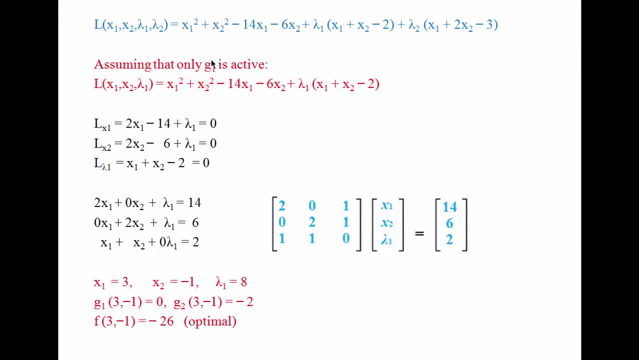 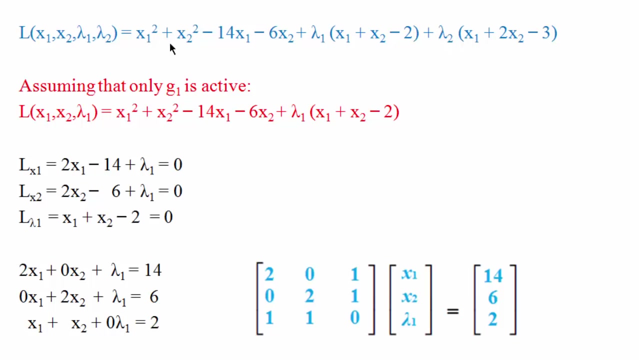 or equal to 0, and since we have positive values here, which means that these values of x1 and x2 are not acceptable for a solution, now let's do another assumption. we are going to assume that only g1 is active, which means that we are going to discard this term and we keep only this equation, which is the 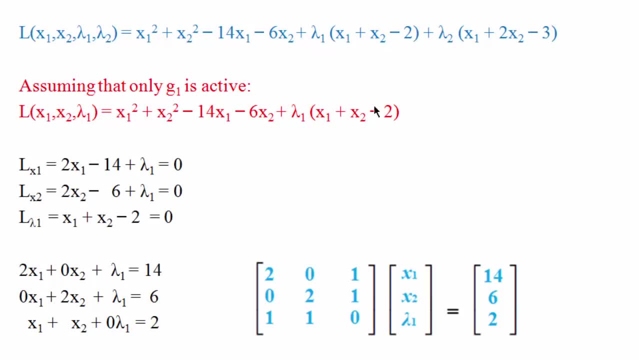 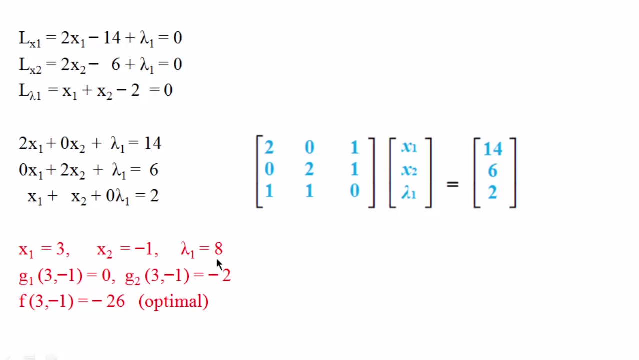 objective function and the first constraint in this equation. similarly, we're going to differentiate with respect to x1, x2 and lambda 1. here we rearrange the equations and the matrix form so we can solve easily to find x1, x2 and lambda 1. now let's test the values by substituting: 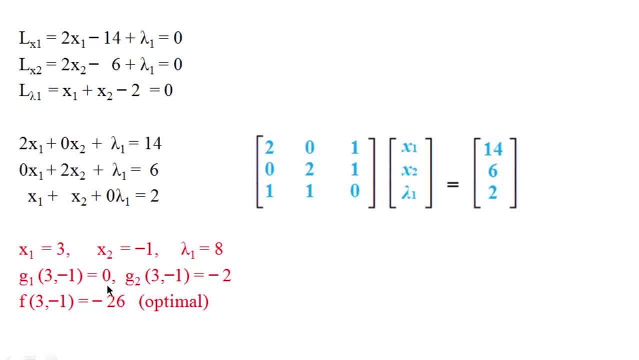 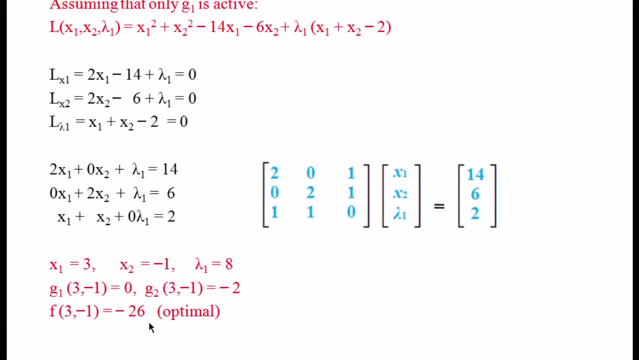 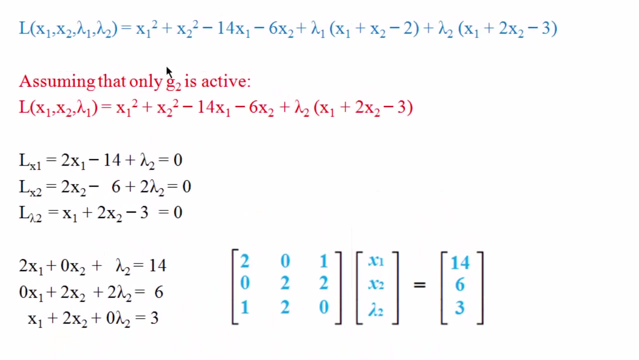 in g1, which gives 0, which is acceptable, and g2 is minus 2, which is also acceptable, and by substituting in the objective function, we get the optimal result, which is minus 26. we can make one further assumption by assuming that only g2 is active. therefore, we are going to discard this term and we'll keep this in. 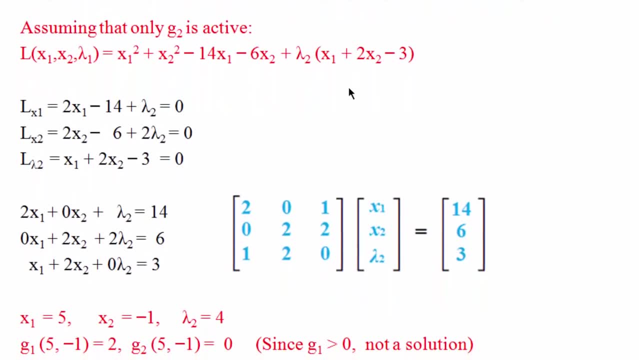 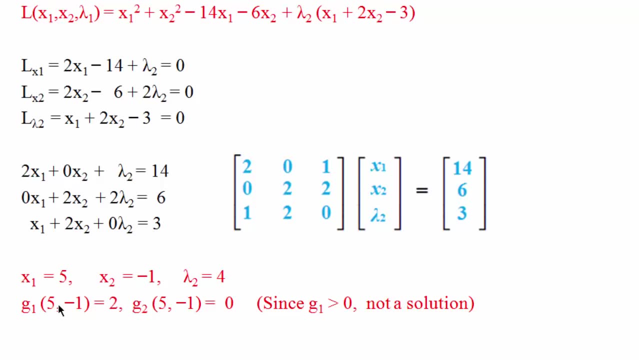 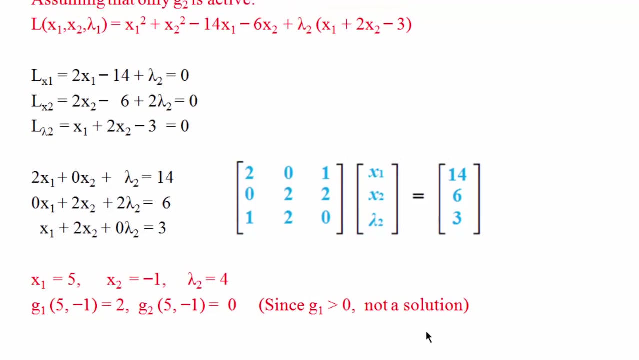 the equation. now we are going to follow the same steps to find x1, x2 and lambda 2 and by substituting we get g1 equals 2 and g2 equals 0. g1 is positive. therefore, we cannot accept it as a solution because if we go back to the previous slides and see the 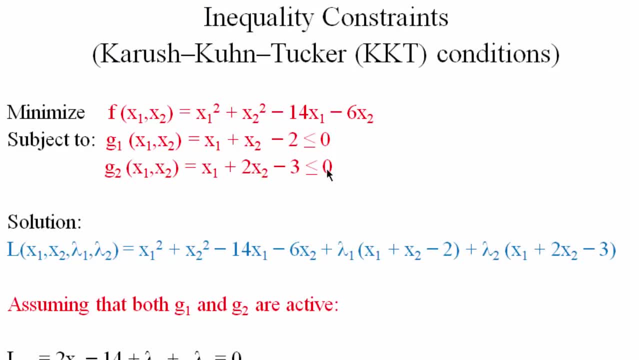 constraints should be less than or equal to 0. so when we have g1 equals 2, for example, positive 2, this means that 2 is less than or equals 0, which is not true. therefore, the value of g1 and g2 should be 0 or negative for. 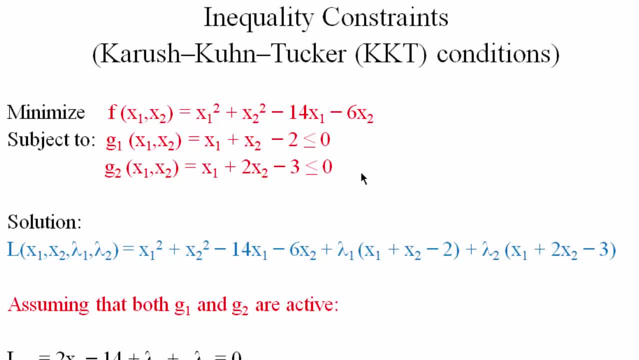 these two constraints to be correct. thank you very much.